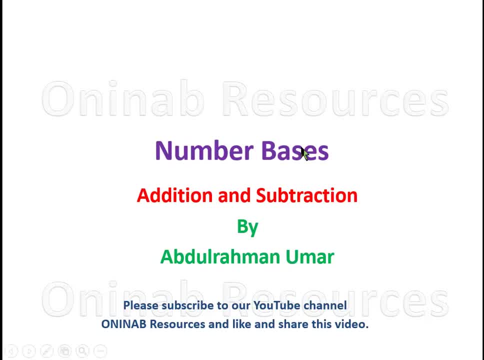 Hello, welcome to another tutorial on number basis. This time around, we will be taking you on addition and subtraction. I still remain Abdurrahman Umar And we still remind you to subscribe to our YouTube channel, if you have not, and enjoy more of our videos. Thank you. 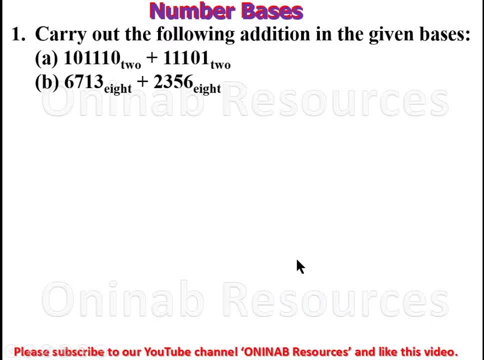 And here we go. Carry out the following addition: in the given basis, We have a 1 0, 1 1 1 0 base 2 plus 1 1 1 0 1 base 2.. So we are going to arrange in a tabular form. Here we go Now. 0 plus 1 gives a 1.. 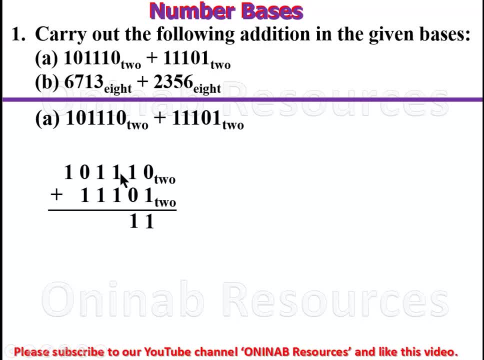 1 plus 1 gives a 1.. 1 plus 1 gives a 1.. 1 plus 1 is 2.. That 2 cannot be written directly, So we are going to convert it to base 2.. So we say 2, divide by 2. We are dividing by 2 because we are working with base 2. And it goes one time and remainder 0. So we are going to carry this 1 and write down this 0. So we write 0. 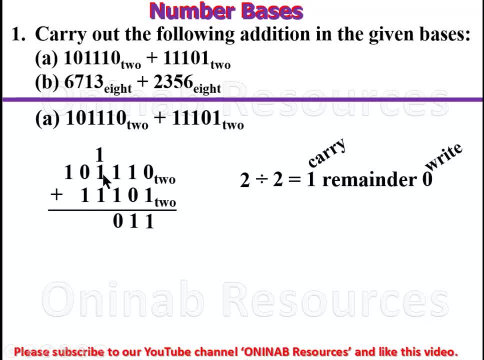 And carry 1.. Now 1 plus 1 gives 2 plus 1 gives 3.. Again we convert the 3 to base 2. So we divide by 2.. It goes one time and remainder: 1. Again we are carrying 1 and writing this 1.. 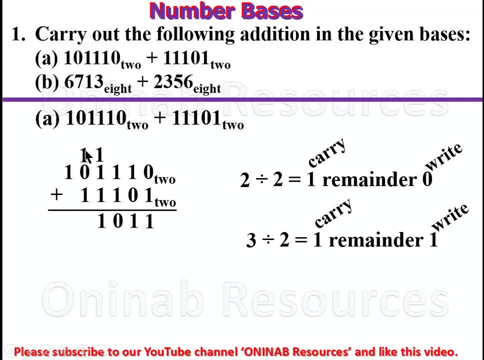 So we write 1. And carry 1.. So 1 plus 1 gives 2.. So this is here And carry 1.. And here again we carry 1 and write 0.. So we write 0 and carry 1.. 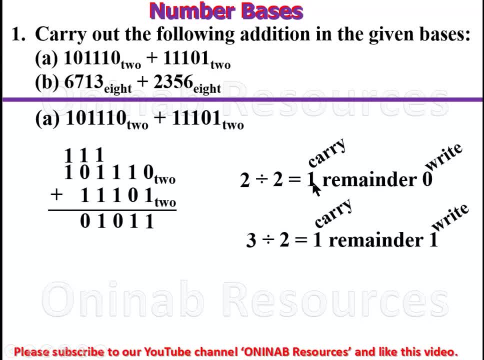 1 plus 1 gives 2 again. So we are carrying. We divide by 2 plus 1 gives 0.. We write 0 and carry 1.. Here we just bring down the 1.. So you have 1, 0, 0, 1, 0, 1, 1 base 2.. 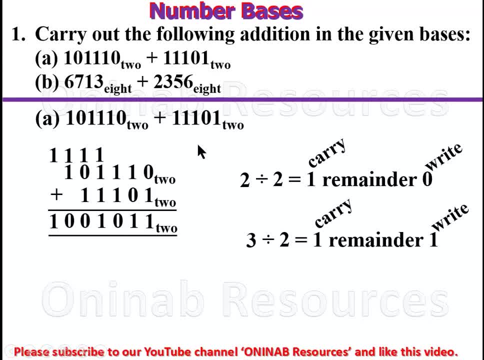 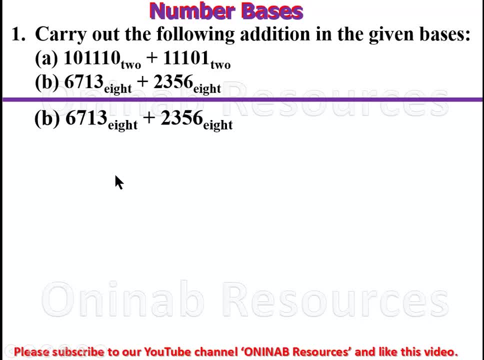 That's the sum of the two binary numbers. So we go to the B part of the problem. So here again we arrange in a tabular form. So we have this. You have to be mindful of this arrangement. This last digit corresponds with the last digit. 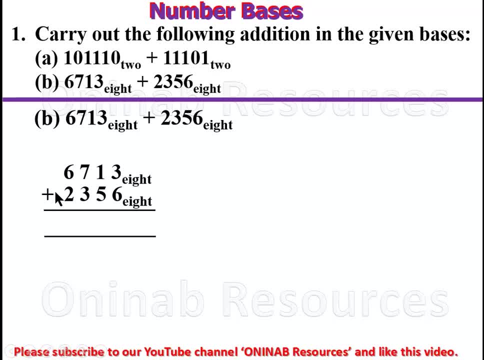 And that's order. So here now we carry out the addition again: 3 plus 6 gives 9.. So 9 is not 1 of the 2.. So we carry out the addition again: 3 plus 6 gives 9.. So we, 9 is not 1 of the 2.. 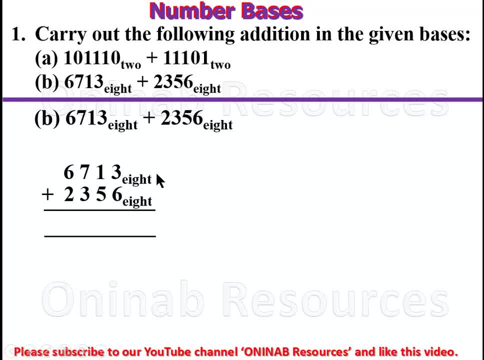 So we carry out the addition again. 3 plus 6 gives 9.. So we 9 is not 1 of the 2. We have the digits of octal number, So we convert the 9 to base 8. So we have 9 divided by 8.. 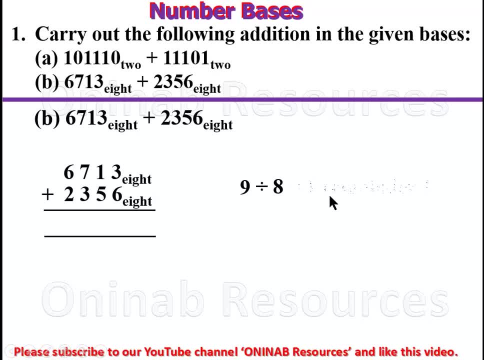 Since we are working with base 8. We are dividing by 8. It goes: one time remainder: 1.. It goes, one time remainder: 1.. So here we carry this: 1. We carry the equations And write down the remainder. 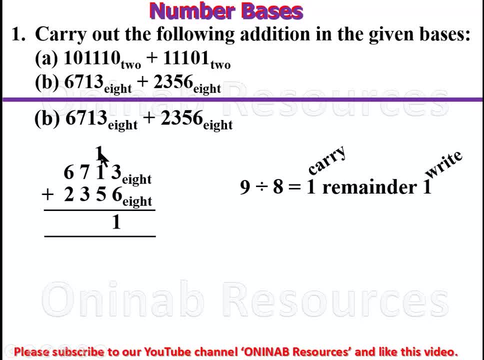 So the remainder is 1. So we carry this. 1. So 1 plus 1 gives 2. Plus 5. gives 7, so we have 7. 7 plus 3 gives 10, so we say 10 divided by 8, which gives 1. 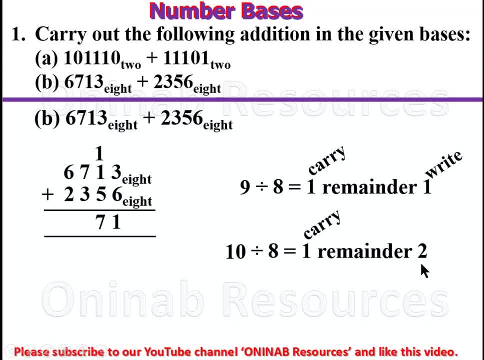 remainder 2. so we are carrying 1 and writing down the 2. so we have 2 and carry this 1. 1 plus 6 gives 7 plus 2 gives 9. again, 9 divided by 8 is 1 remainder 1. so we are writing this 1 and carry the 1. so since there's no, 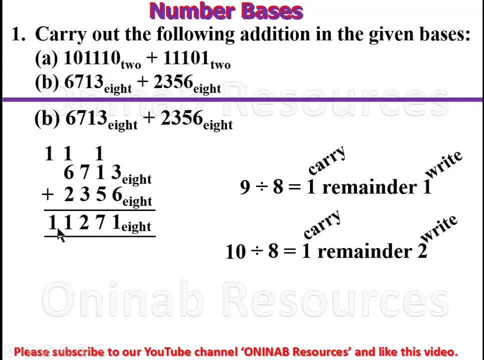 number to add the 1 to. we just bring down the number and we have 1, 1, 2, 7, 1 base 8 as the result of the sum of this octal number. so this method is the same with respect to any base you are working with. so we now go to the second problem. 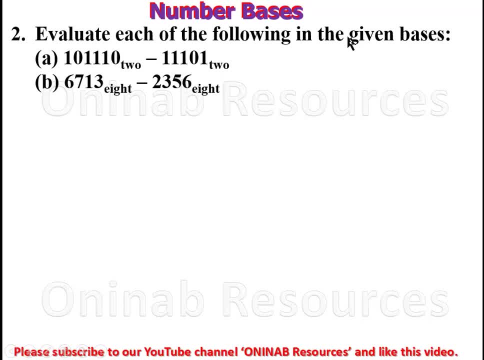 the second problem is the following: we are to evaluate each of the following in the given basis. so we have the problem A. so again, we arrange the tabular form and please be reminded: 1, 2, 3, 4, 5, 6. we have 6 digits here and 1, 2, 3, 4, 5, and we have 5 digits here. so we 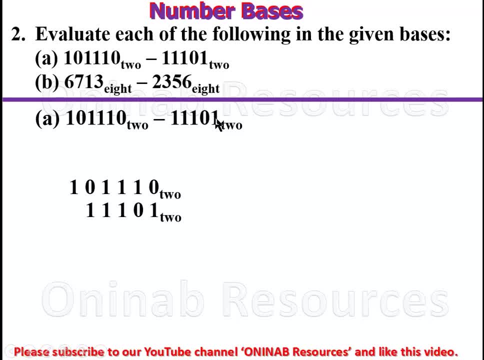 arrange it in such a way that the last digit correspond with the last thing, the second to the last digits correspond with the second to the last digits, and so on. so we carry out this subtraction. now we cannot say 0 minus 1, so that will be impossible here. so we borrow this one. we borrow this one and it will be left. 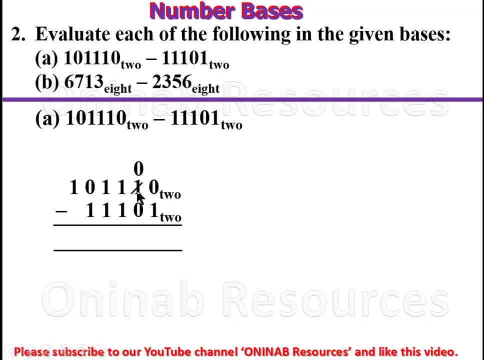 with 0 here. when we borrow- since we are working with base 2, what we borrow is 2, so we have the 2 here and we have 2 here, and we have 2 here and we have 2 here, and 2 minus 1 gives 1. we are now left with 0. 0 minus 0 gives 0. 1 minus 1 gives 0: 1 minus. 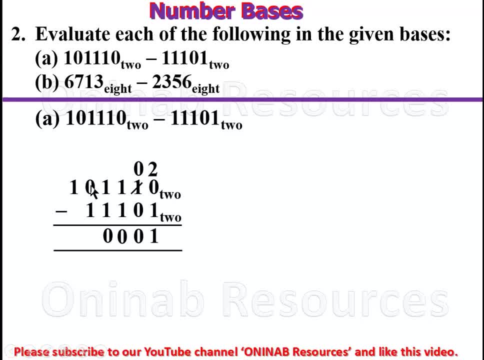 1 gives 0. again, it's not possible to say 0 minus 1 in base 2. what we do is to borrow this one and it will now be 0 there. bringing it here is 2, because the base we are dealing with is in base 2. so 2 minus 1 gives a 1 in base 2.. 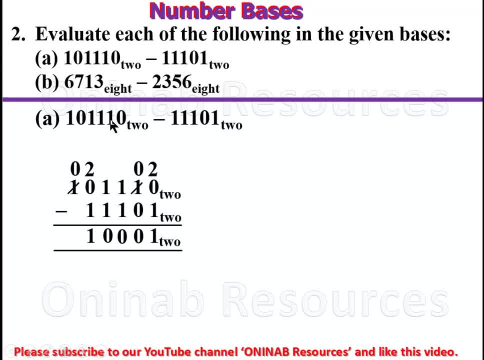 this is the result of the difference between these numbers in base 2. so we go to problem b. we have a 6713 base 8 minus 2, 3, 5, 6 base 8 and we arrange again in a tabular form. so we are going to. we now carry out the subtraction. 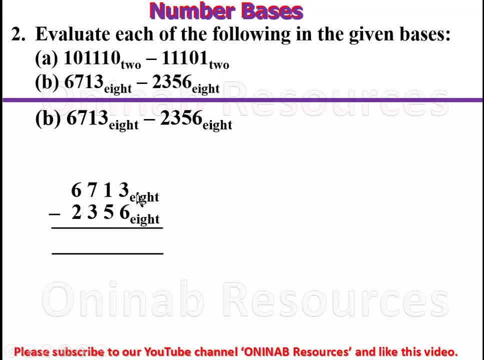 out the subtraction Here. we are working with base 8 and it is not possible to say 3-6 in base 8 here, So we borrow this: 1. We are left with 0 there. Bringing it here. it is 8 because